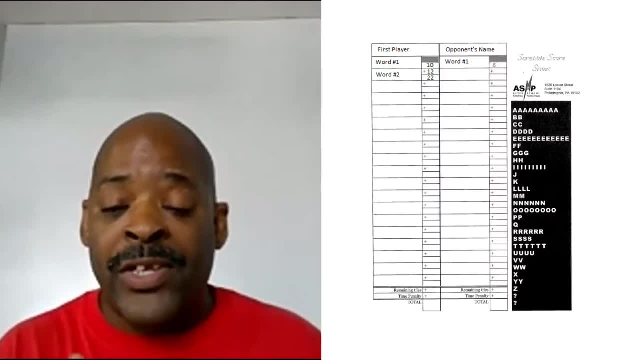 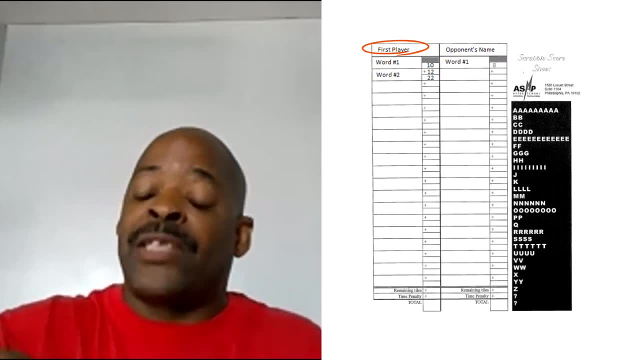 who goes first. their name always go on the top of the left-hand side of the score sheet. That means, if you got the closest letter to A out of the bag and you're first, your team's name or your solo name will go on the left-hand side. Your opponent's name will then go on the right-hand. 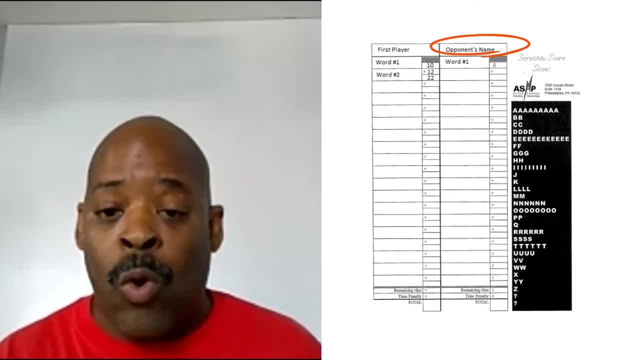 side. Now also when you're keeping score. once you have your name down, Pat, now first word say: it's man M-A-N and you have 10 points for man. you will put that in the first. 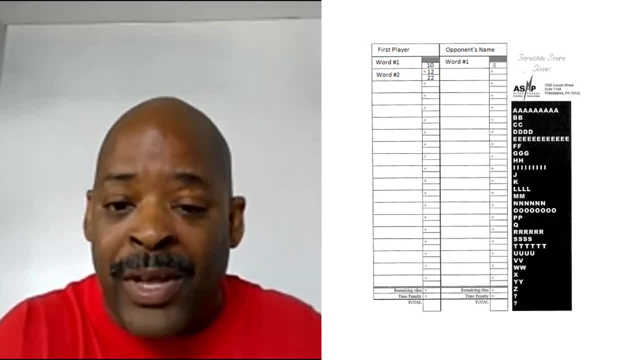 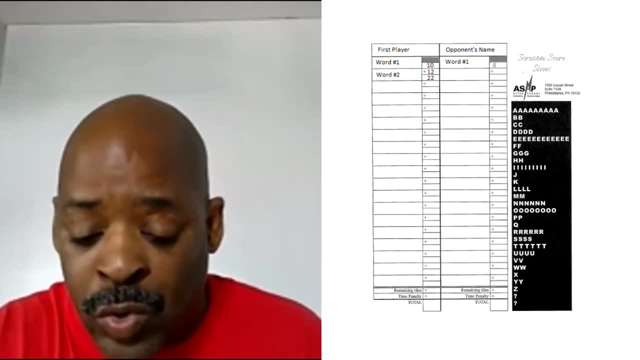 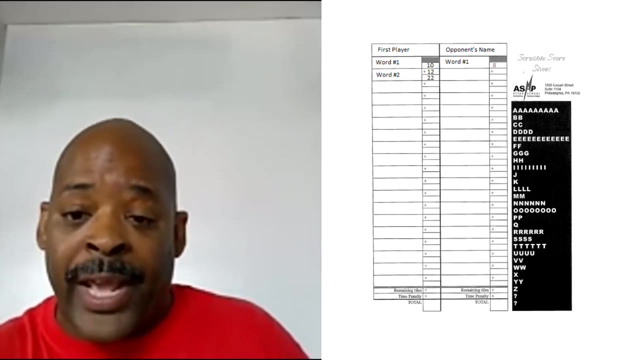 column And over to the little side where you see the plus sign, you will put the amount. So, man, you write man in there. you score 10 points, you go to and you write 10.. Now your opponent is second. they put their name down, they put their score down and the amount they have in. 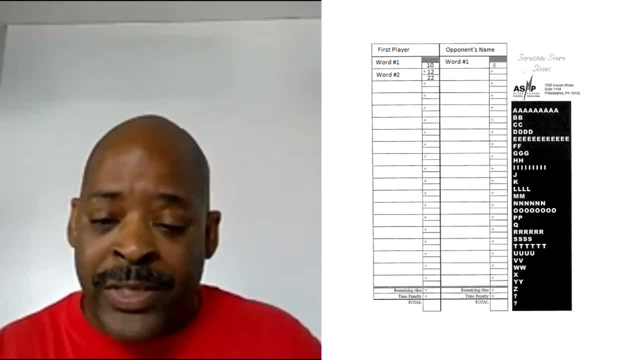 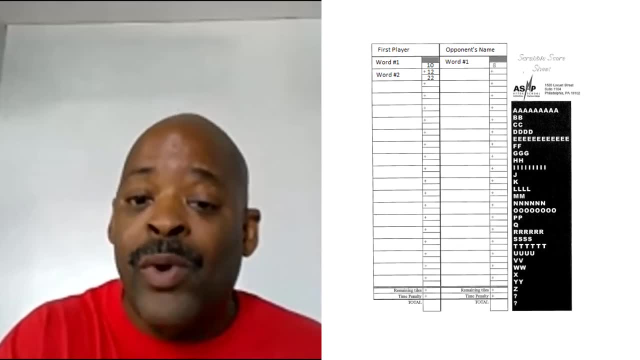 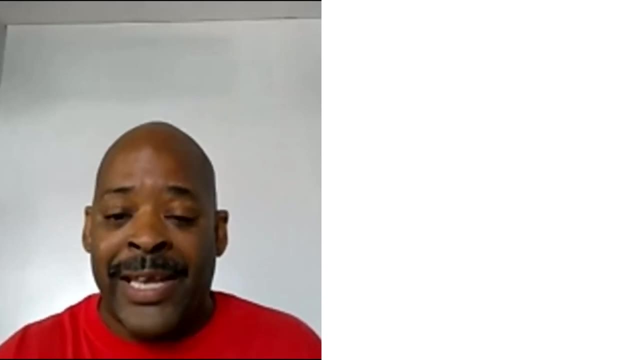 their little box. Now, when you go again, you score 10 points. Now say you score 12 points, You put your word down, you put the 12 under the 10, and then you add it up: 10 plus 12 equals 22.. And you add this up all the way down to the end of. 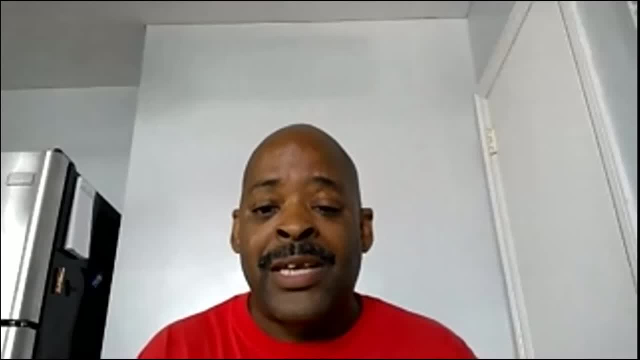 the game. This stops from discrepancies in the score sheet. If there's a problem with the score, you can always find out if you keep score this way. Now. if you're skipping scores and not putting the score down, that's fine. You can always find out if you keep score this way. Now, if you're. 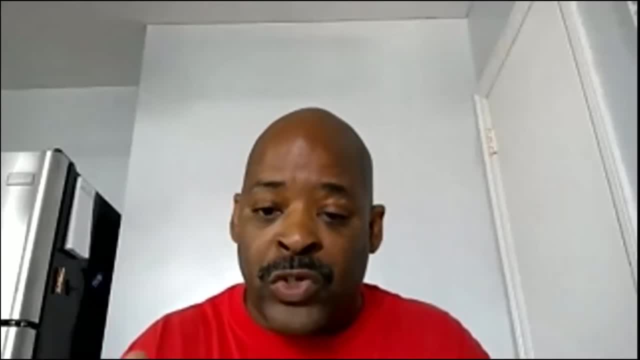 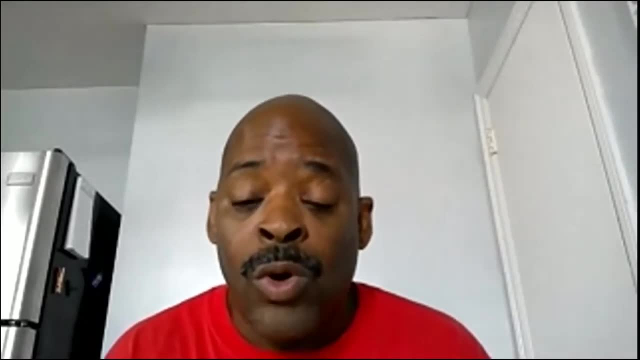 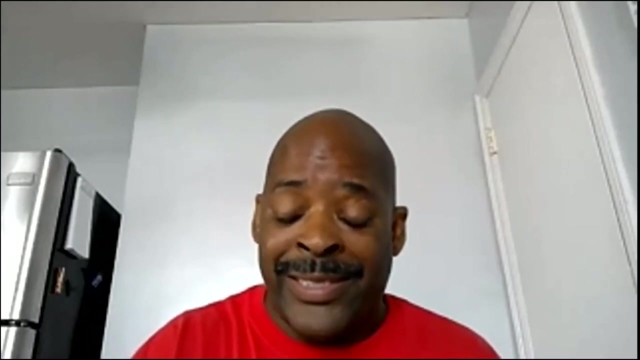 going to be a disaster. So always remember to put your word down and put the score down as soon as after you put the word on the board. So on the Scrabble board the most important is triple word score. Then you have double word score, You have a triple letter score and you have a double letter. 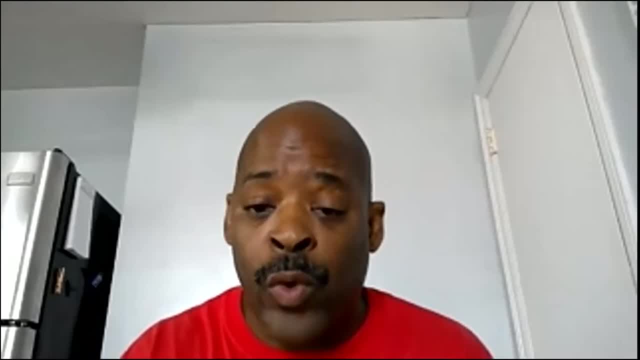 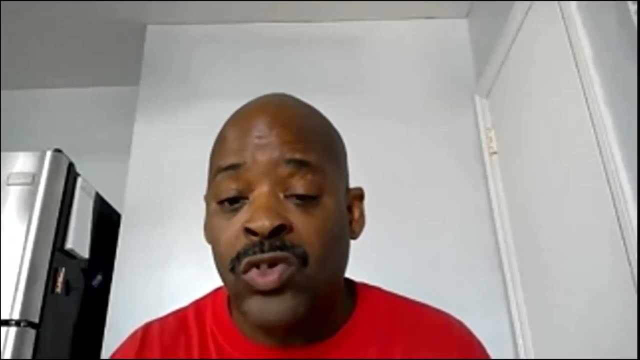 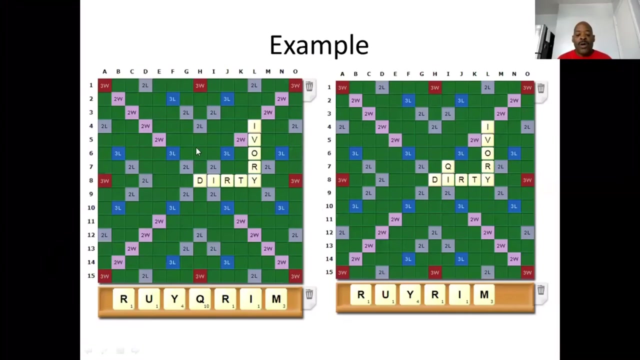 score. These are the most important squares where you could get the most points for your word. But remember, in scoring points you also have to try to play defense, to not let your opponent get the squares before you do. Okay, here's an example: On the board you have dirty.